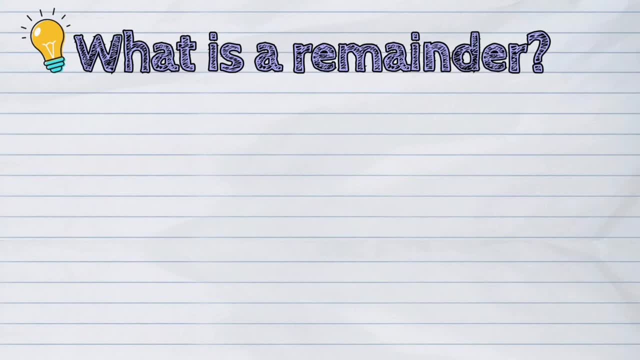 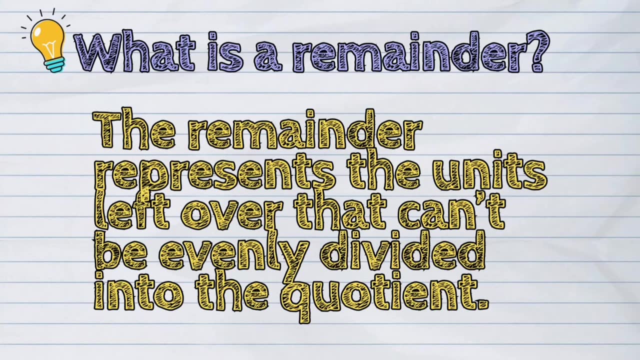 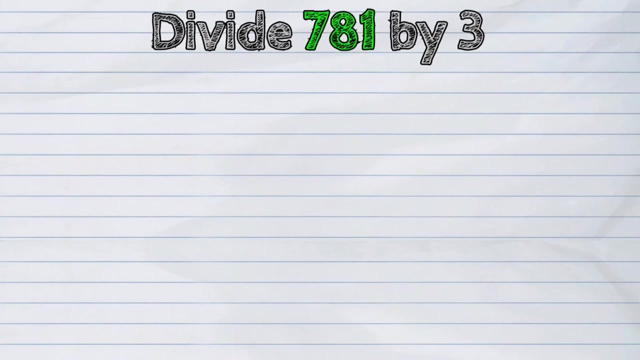 we need to know first the definition of remainder. The remainder represents the units left over that can't be evenly divided And it can't be divided into the quotient. Now let's study this example: Divide 781 by 3.. First we need to arrange the numbers in a division bracket. 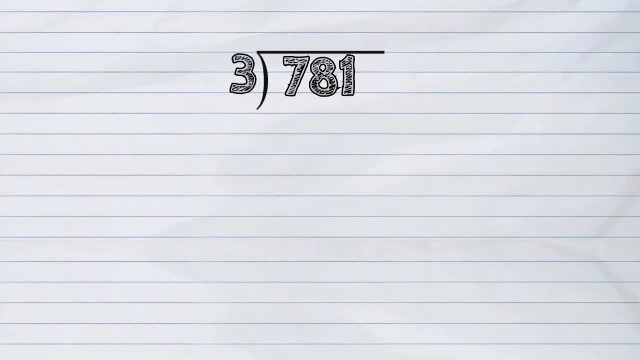 Let us start with the first number of dividend, Which is 7.. This will be divided by the divisor 3.. How many times can we divide 3 into 7?? The answer is 2.. So we should put digit 2 in the quotient line. 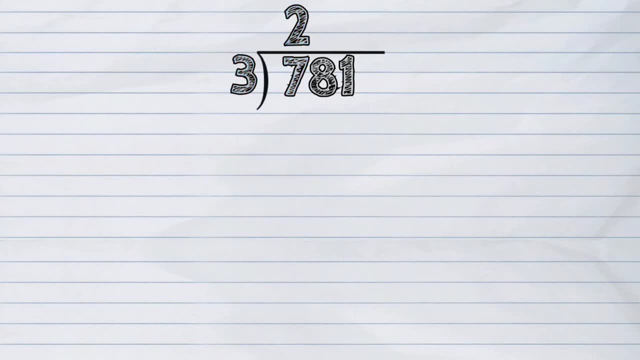 The second step is to multiply. We will multiply our answer from step 1., Which is 2., And our divisor, which is 3.. 2 times 3, the answer is 6.. We write 6 under digit 7.. 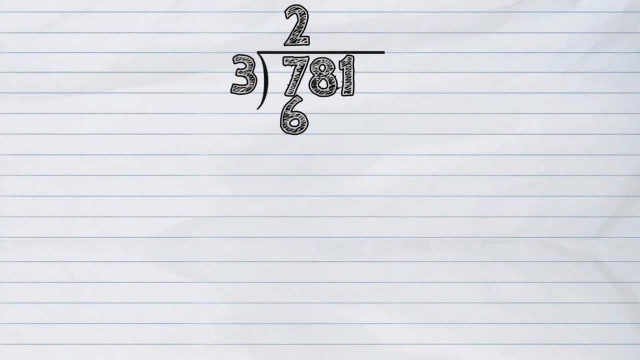 The next step is to subtract. In this case it will be 7 minus 6.. The answer is 1.. The fourth step here is to bring down the next number from the dividend, Which is 8 tenths. We write 8 next to digit 1.. 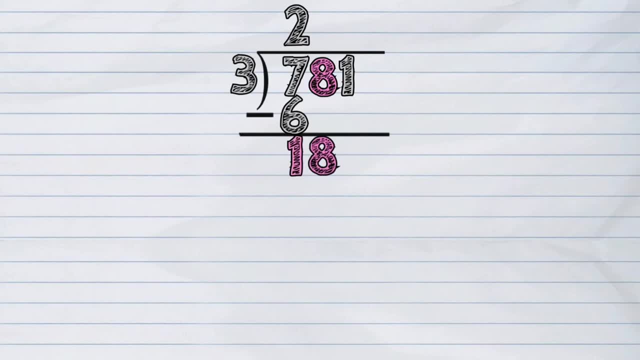 Making the number 18.. Now we will do again the process of step 1. Divide. We will divide 18 tenths by 3. How many times can you divide 3 into 18?? The answer is 6.. 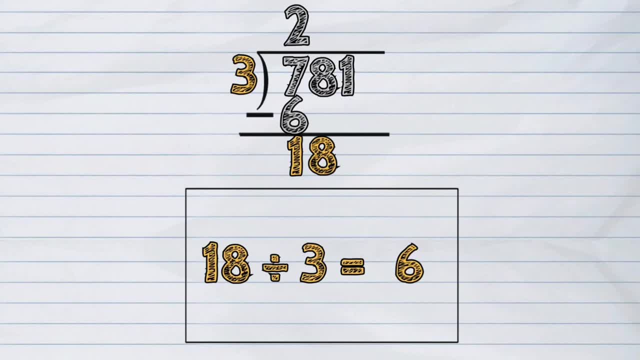 6.. We write the answer next to digit 2.. Next we have to multiply. Multiply 6 into our divisor again, which is 3.. 6 times 3 is 18.. We write the answer below 18.. 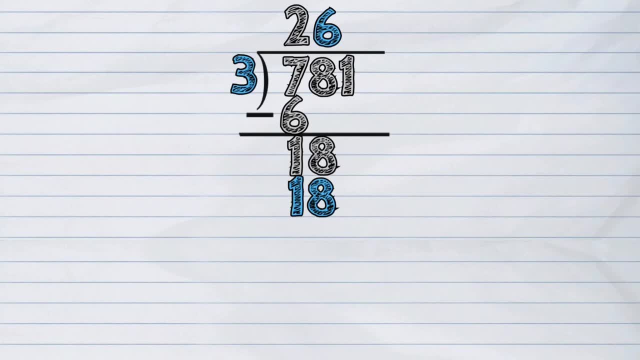 18. 18. 18. 18. 8 times 3.. Then we will do again the subtraction 18 minus 18.. The answer is 0. 0. And then we bring down the next number from the dividend, which is 1.. 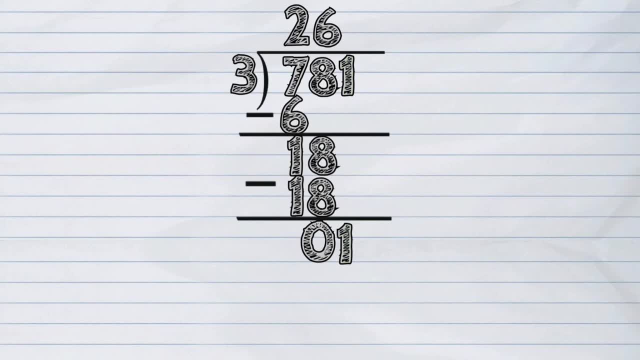 We'll repeat the step 1 process By dividing 1 by 3.. Divide the number again from the dividend, Which is 1.. Divide again from the dividend: Divide 3.. Can we divide 1 by 3? That would not be enough. So what we are going to do is to write down 0 as the answer. 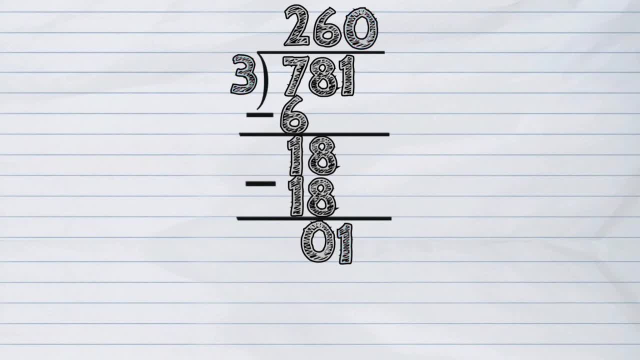 4.. Then multiply 0 and 3. The answer is 0.. Now we subtract 0 from 1,, which gives the answer of 1. 5. As you can see, there is still 1 left over, but no more numbers to bring down. 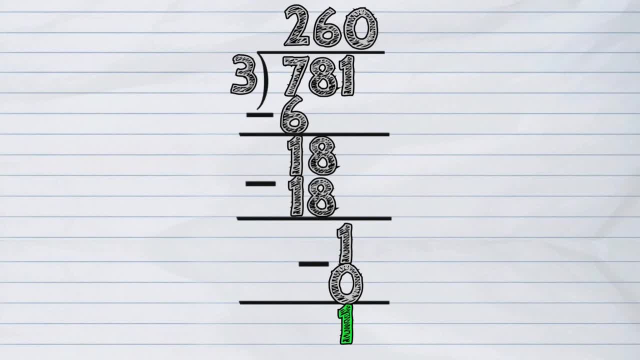 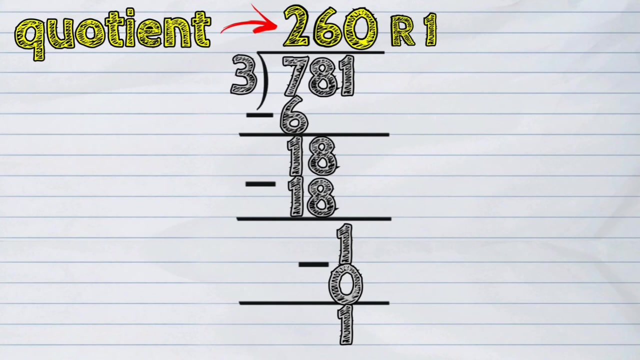 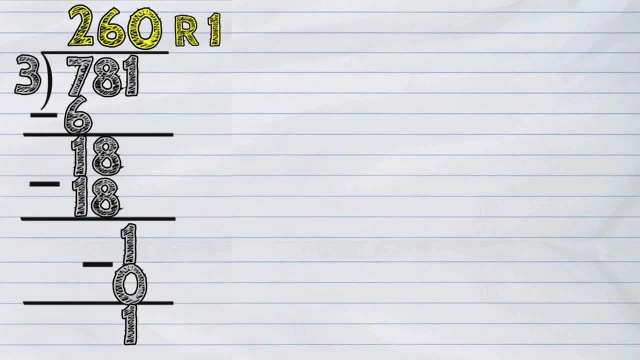 6.. So this will become our remainder. Take note that a remainder must be less than the divisor and is written as part of the quotient 7.. Therefore, the quotient is 260, remainder 1. 8.. We can check our answer by using this formula.